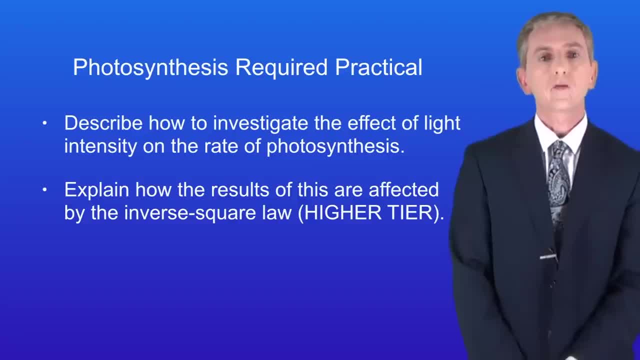 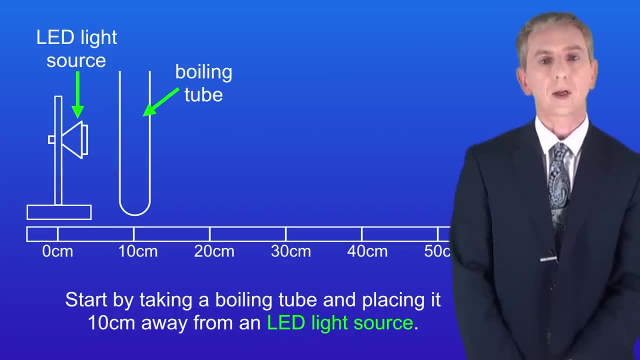 of this are affected by the inverse square law. This is the required practical, so you need to learn the details. We start by taking a boiling tube and placing it 10cm away from an LED light source. An LED light is used, as these don't release very much heat Too. 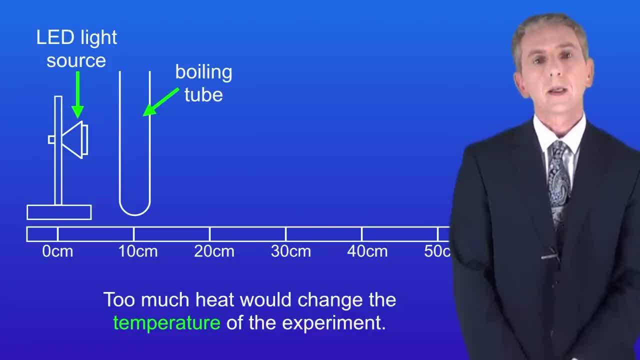 much heat would change the temperature of the experiment. Now, if we have to use a normal light bulb, then we need to place a beaker of water between the light and the boiling tube. This absorbs the heat produced by the bulb. Now we fill the boiling tube with sodium. 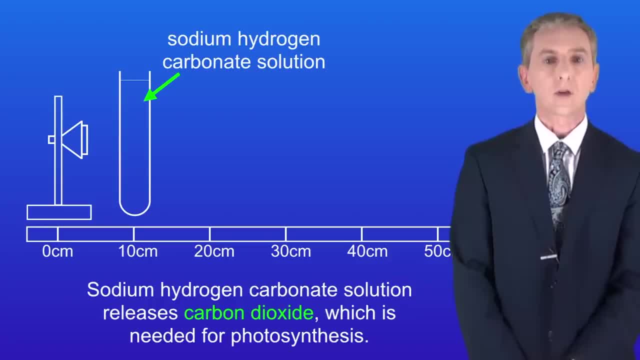 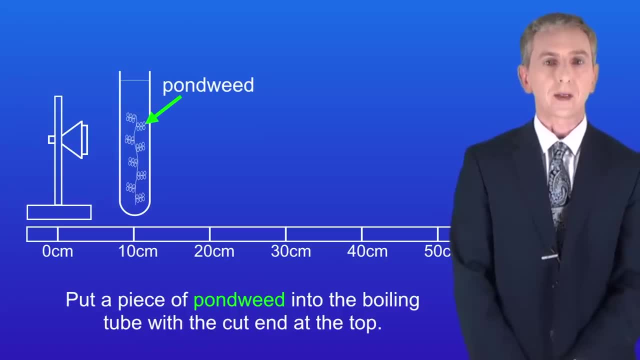 hydrogen carbonate solution. Sodium hydrogen carbonate solution releases carbon dioxide and that's needed for photosynthesis. Next we put a piece of pondweed into the boiling tube with the cut end at the top. We then leave this for 5 minutes to acclimatise to the conditions in the boiling tube. We should see bubbles. 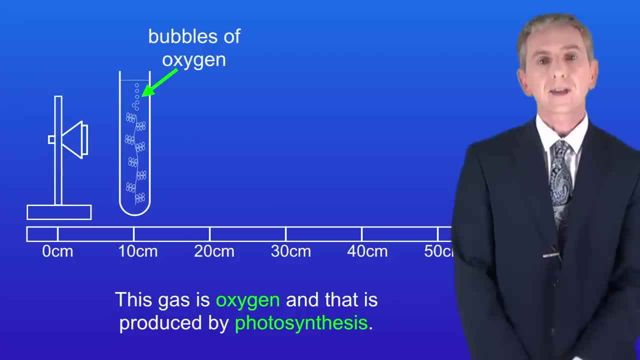 of gas being produced from the cut end of the pondweed. This gas is oxygen and that's produced by photosynthesis. Now we start a stopwatch and we count the number of bubbles produced in one minute. We then repeat this two more times and we calculate the mean number. 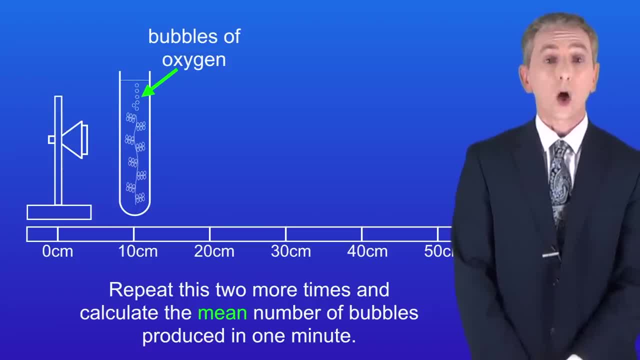 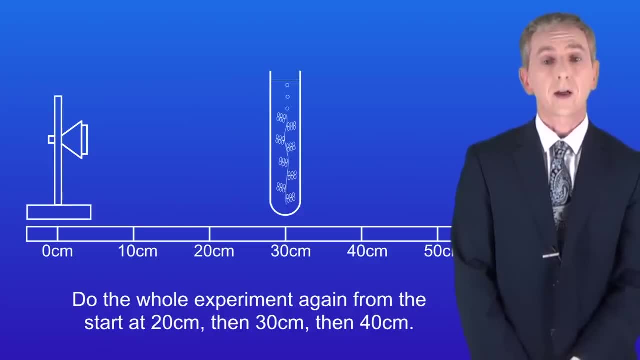 of bubbles produced in one minute. Next we do the whole experiment again from the start, but this time at 20cm, Then we do it at 30cm and finally at 40cm. Now there are two main problems with this practical. Firstly, the number of bubbles. 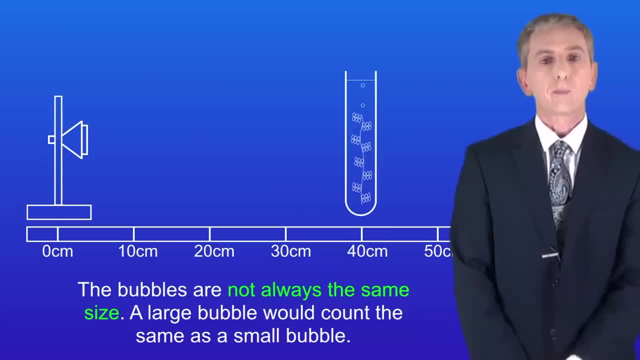 can be too fast to count accurately. Secondly, the bubbles are not always the same size, so, for example, a large bubble would count the same as a small bubble. Now we can solve these problems by measuring the volume of oxygen produced instead of counting bubbles. 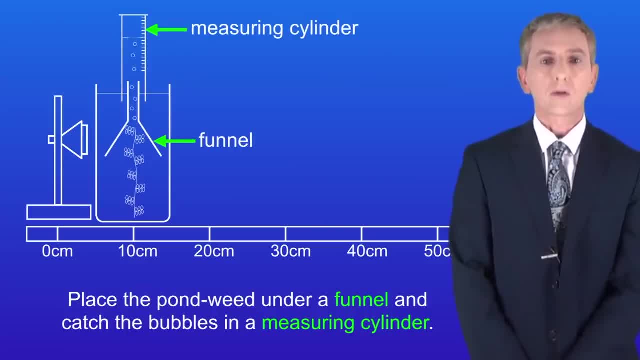 We use this equipment. We place the pondweed under a funnel and we catch the bubbles in a measuring cylinder filled with water. We then use the measuring cylinder to measure the volume of oxygen produced. Now, if you're a foundation tier student, you can stop watching. 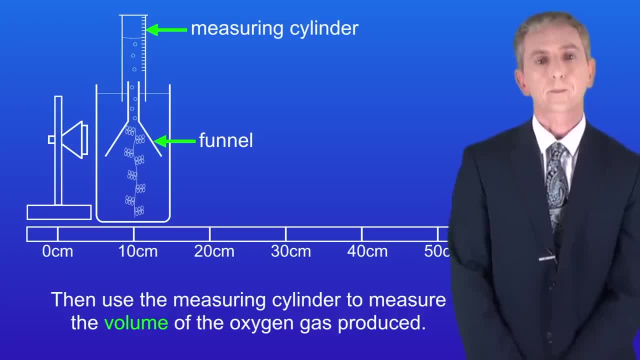 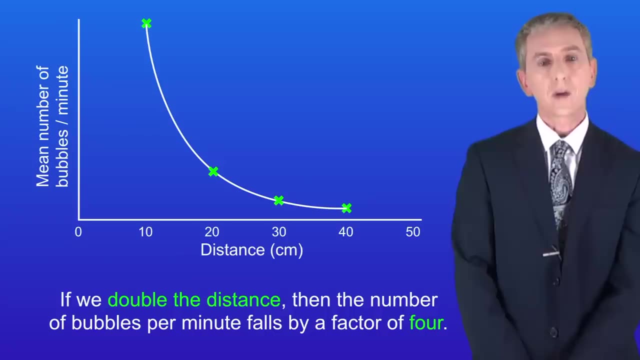 now, However, higher tier students need to continue watching. If we plot the mean number of bubbles per minute or the volume of oxygen per minute against the distance from the lamp to the pondweed, then we get this graph. Now, the key point about this is that if we double the distance, then the number of bubbles per